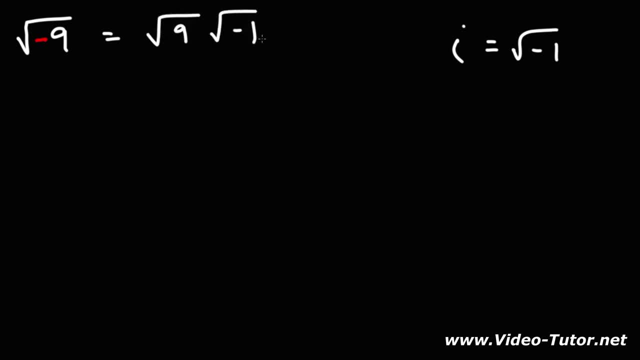 into the square root of nine times the square root of negative one, because nine times negative one is negative nine. Now the square root of nine. we can make that three and the square root of negative one. that becomes i. So three times i is simply three i. So that's the answer for this. 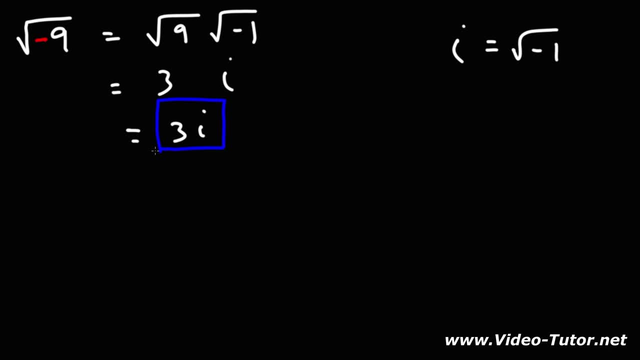 problem. That's what we can evaluate, the square root of negative nine. Now let's try some other problems. Feel free to work on these two example problems. if you want to Take a minute, pause the video and try this problem as well as this one. 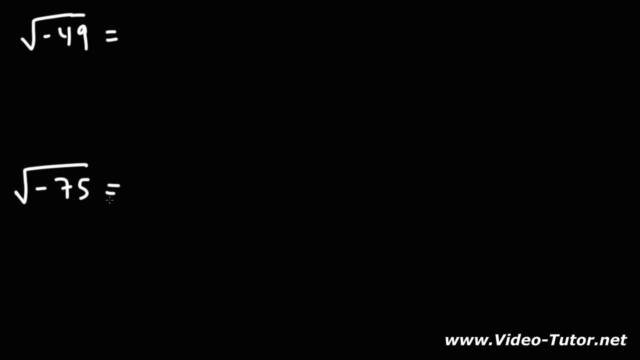 Now the square root of negative 49, we can write that as 49 times negative one, And we know the square root of 49 is seven because it's a perfect square. Seven times seven is 49. And the square root of negative one is i, So this becomes seven. Now what about the square root of negative 75?? 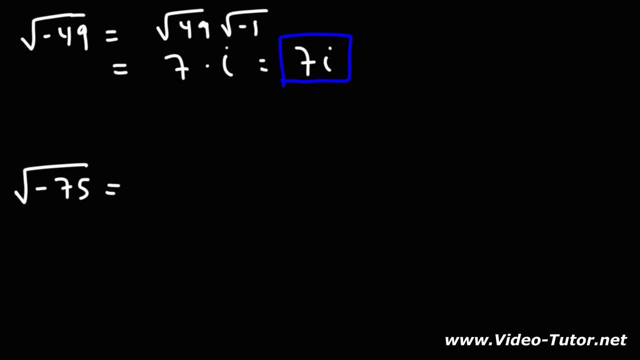 What can we say for that one? 75 is not a perfect square like four, nine, 16,, 25, or 49.. However, three times 25 is 75, and 25 is a perfect square. So what we want to do is we want to break. 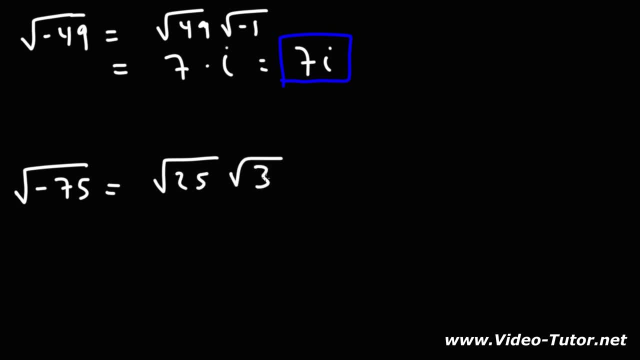 down 75 into 25 and three, because 25 is the highest perfect square that goes into 75. So we're going to have this: The square root of 25 is five. The square root of negative one is i, So it's simply five root three times i. Now let's try another problem like that. Go ahead and simplify. 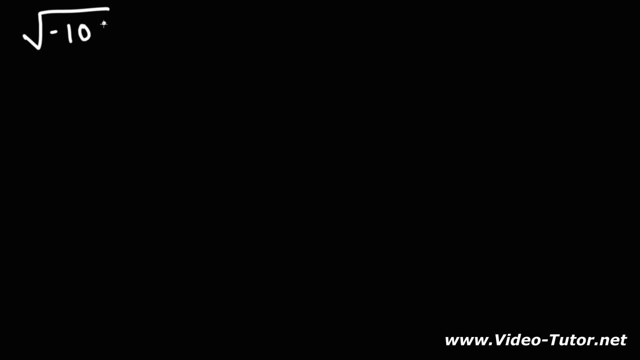 this one Square root negative 108.. And also negative square root negative 80.. So, in order to simplify the square root of 108, we want to find the highest perfect square that goes into 108.. So the perfect squares that we know are: one: two squared is four. three squared is nine. 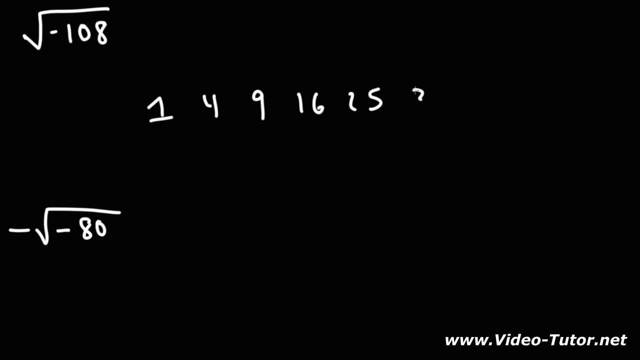 four squared is 16,, five squared is 25,, six squared is 36,, seven squared is 49,, eight squared is 64.. So what's the highest perfect square that goes into 108?? The answer is 36.. 36 times three is 108.. 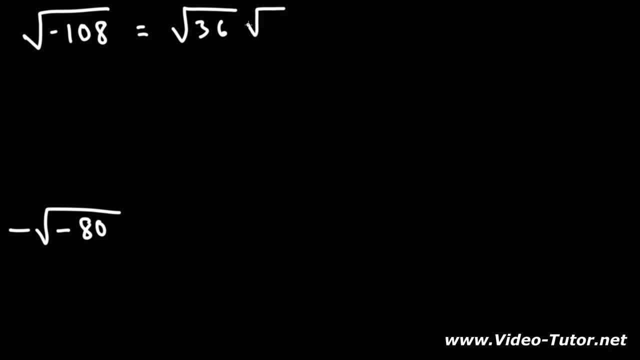 So we can write this as: the square root of 36 times the square root of three times the square root of negative one. The square root of 36 is six and the square root of negative one we know it to be i, So our final answer is going to be six square root three times i. 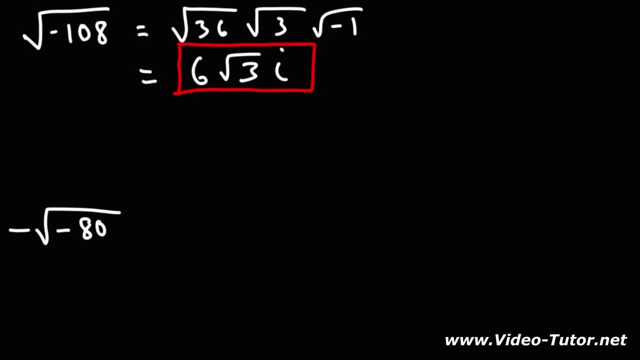 Now for the next one. we need to find the highest perfect square that goes into 80,, which is going to be 16.. 16 times five is 80. So what we're going to have is 16, five and the square root of negative. 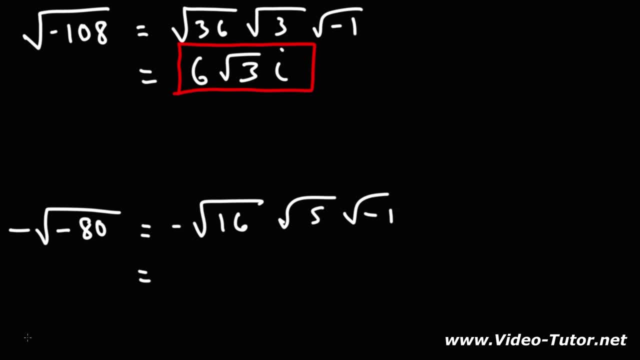 one. So the negative on the outside, that's going to stay there. So we're just going to keep it here. So we have negative. the square root of 16 is four and then times the square root of five, and the square root of negative one is i. So this is going to be negative. four root five times i. 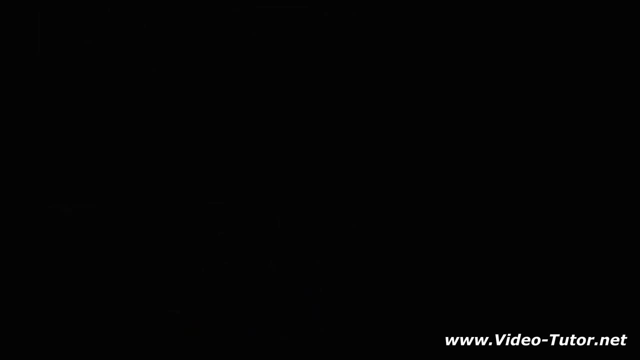 There's a train passing by Now. let's say if we have this quadratic equation: x squared plus 18.. I'm going to draw a better: eight x squared plus 18 is equal to six. x squared plus 18 is equal to zero, and we're tasked with the assignment to solve for x. 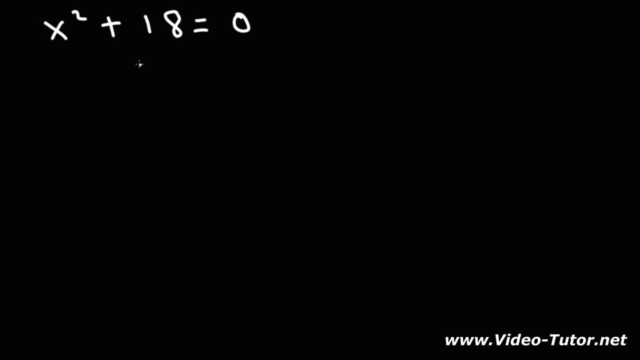 How can we do that? The first thing I would do in this problem is I would subtract both sides by 18.. So 18 and negative 18 will cancel out. I could bring down x squared and zero plus negative 18 is negative 18.. 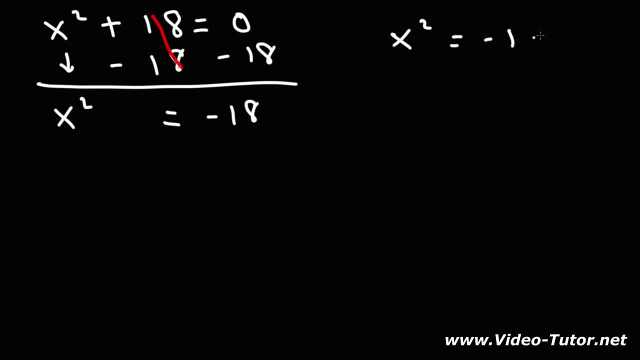 So I get x squared is equal to six. So I get x squared is equal to negative 18.. Now, in order to get x by itself, in order to solve for the value of x, I need to go ahead and take the square root of both sides. 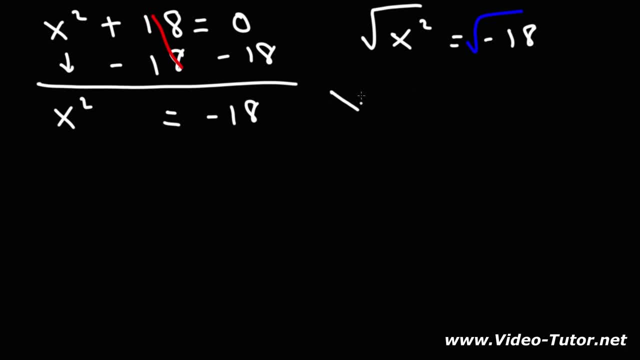 The square root of x squared is x. What about the square root of negative 18?? Whenever you take the square root of x squared, you're going to get two possible answers. So it's going to be plus or minus, and then the square root of negative 18..